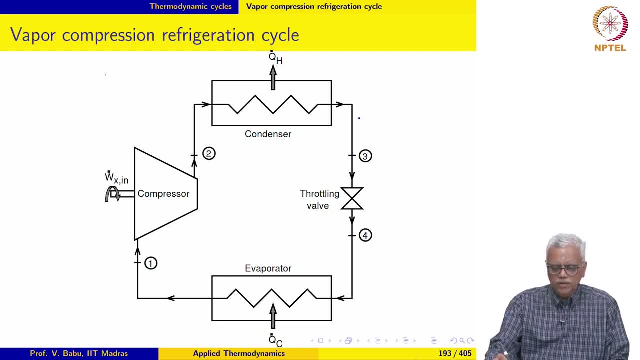 cycle is a power absorbing cycle, And what we are going to discuss today is the cycle that is used in domestic refrigerators and domestic air conditioners. This was discussed in detail in the previous course, So for those of you who have not gone through that, 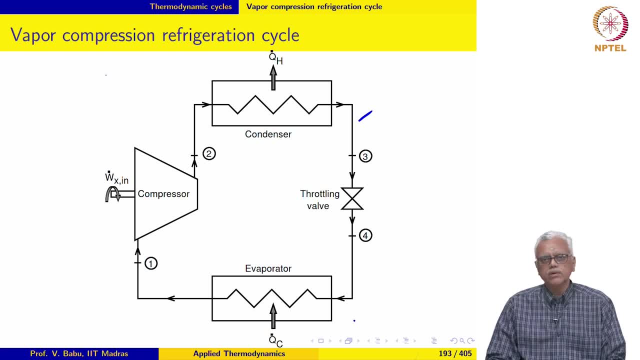 material. I suggest that you go through this module on vapor compression cycle in the previous lecture, But we will quickly recap whatever was said there. So basically we start at state 1 here where the refrigerant, So here the refrigerant. 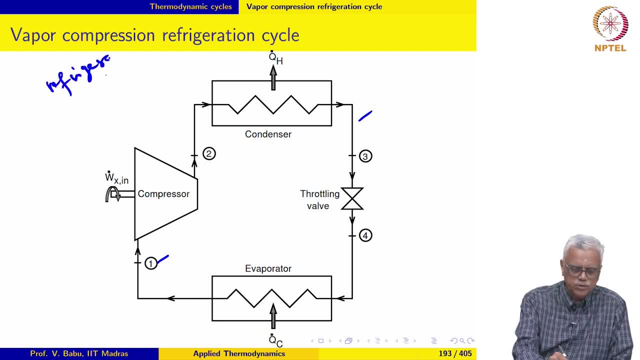 is the working substance. So, similar to the Rankine cycle where water was the working substance and it remained as water throughout the cycle, Here refrigerant is the working substance and it remains as refrigerant throughout, unlike the air standard cycles where the air 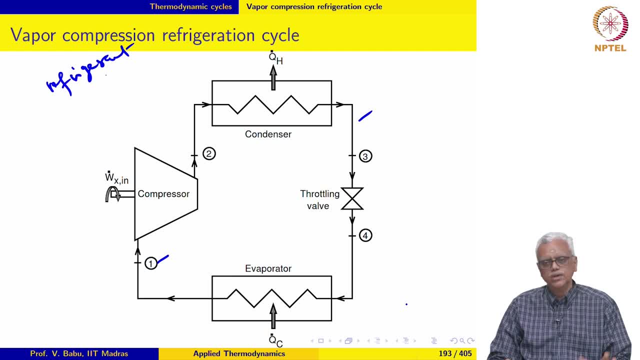 was taken in. This is because air is mixed with fuel and burned, So you have air coming in and then combustion gases leaving, So the working substances does not execute a cyclic process there. In this case, the refrigerant is the working substance and it executes a cyclic. 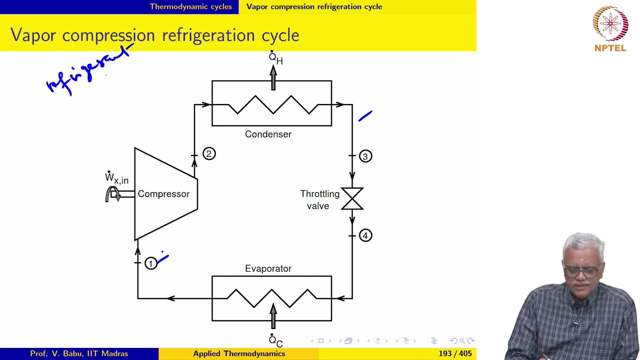 process. So let us start with state 1.. So state 1 is entry to the compressor. So here the working substance is at low pressure and relatively low temperature, So the air starts from the 부 있고요. 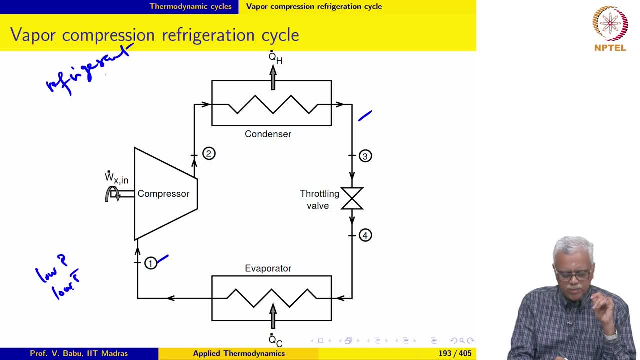 relatively low temperature, and it can be a saturated vapor or slightly superheated also, it does not matter, let us write it down as saturated vapor. So that is the thermodynamic state at state 1.. So the refrigerant then enters the compressor, where it is compressed to high pressure, high. 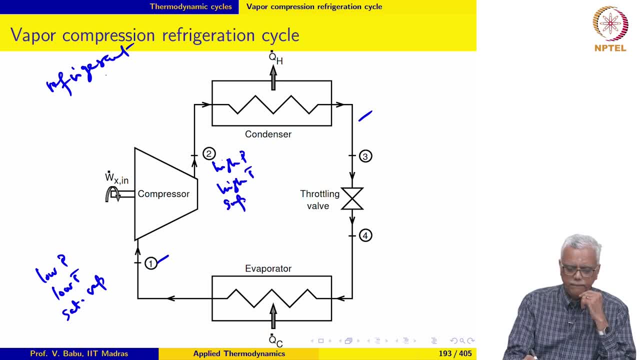 temperature and superheated. So the high pressure, high temperature refrigerant is then sent to the condenser where it loses heat with the ambient. So if you look at, say, slightly older refrigerators, you should be able to see the cooling coils at the back of the refrigerator. 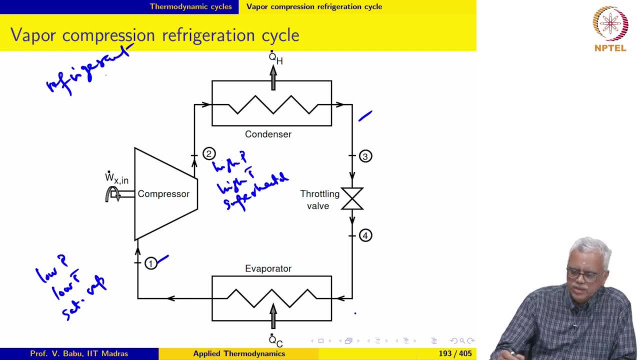 So that is the condenser, where the refrigerant loses heat with the ambient. So as it comes out of the condenser, the refrigerant is at a high pressure, reasonably high temperature, not very high, Reasonably high temperature, and it actually usually comes out as a saturated liquid, although 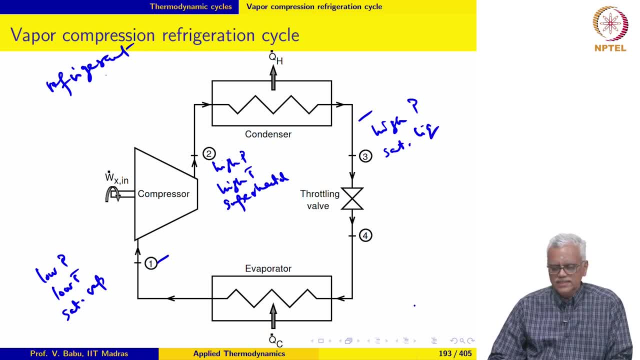 this need not exactly be the case, but for now let us take it as saturated liquid. Now the refrigerant is then throttled in the throttling valve, So the high pressure, reasonably high temperature refrigerant now comes out as low pressure, low temperature saturated mixture. 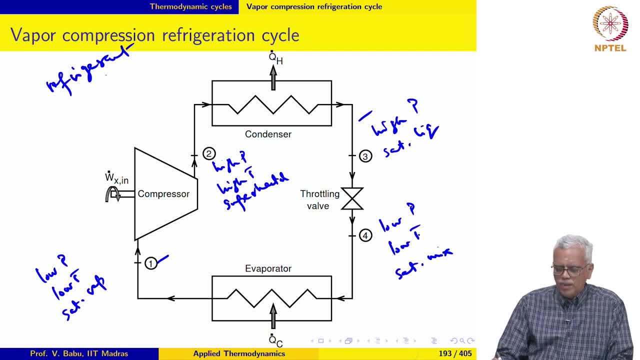 So the temperature of the refrigerant. So the temperature of the refrigerant drops as a result of throttling and it then enters the evaporator. So this is the refrigerated compartment or the air conditioned room. So the refrigerant, then the cold refrigerant, picks up the heat from the refrigerated compartment. 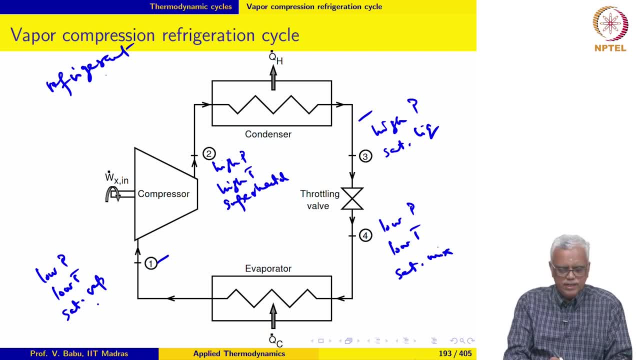 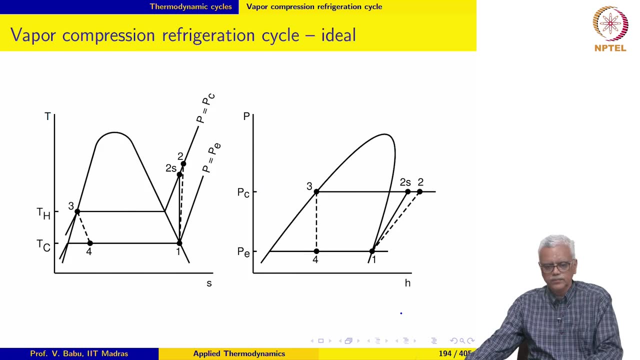 and as it picks up the heat, it undergoes change of phase, and then it goes from being a saturated mixture to a saturated vapor, and the cycle is repeated. Okay, Okay, Now we may illustrate the cyclic process executed by refrigerant on a T-S diagram, or: 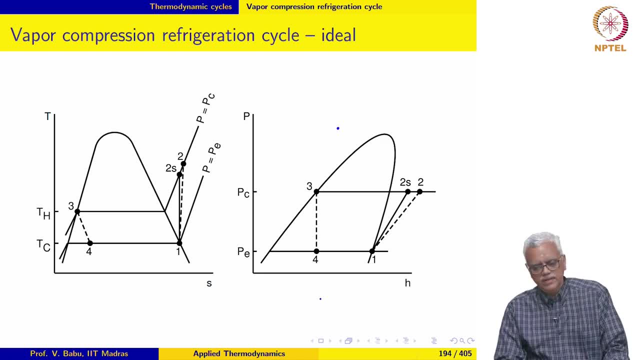 on a P-H diagram. I will come to the P-H diagram next. Let us first look at the T-S diagram. So, just like the Rankine cycle or the Brayton cycle, the vapor compression refrigeration cycle also operates between two isobars: P equal to Pc, which is the condenser pressure. 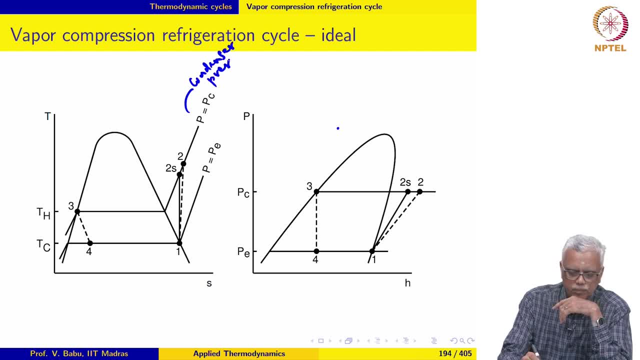 Okay, Okay, Okay, Okay, Okay, Okay, And P equal to Pe, which is the evaporator pressure. Okay, So, state 1, we have taken it to be a saturated vapor. So saturated vapor at evaporator pressure. So it enters the compressor, where it is compressed from state 1 to 2s in case of an isentropic. 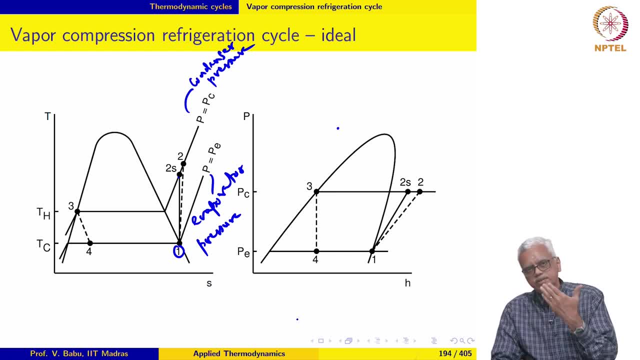 compression. Okay, So in the situation where we allow for internal irreversibilities in the compressor, the end state will be state 2.. So you can see that the state corresponding to 2 is high pressure, high temperature and superheated, as I mentioned before. 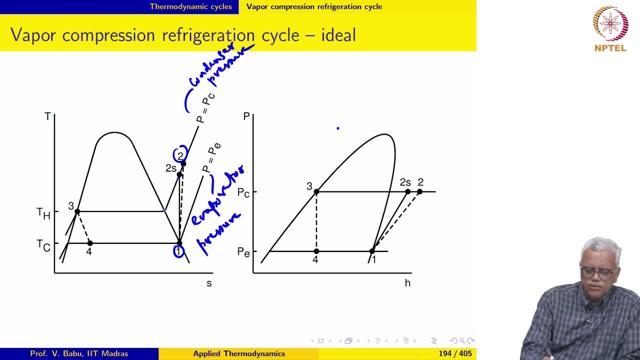 So it is then taken to the condenser and it loses heat to the ambient at constant pressure, undergoes change of phase starting from here And the fluid leaves the condenser as a saturated vapor. Okay, So it leaves the condenser as a saturated liquid at condenser pressure. 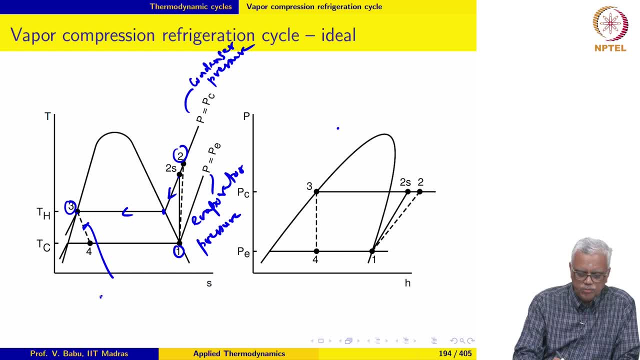 So it is then throttled in the throttling valve. So this is the throttling process. So it is throttled to a low temperature, low pressure, saturated mixture and it then enters the evaporator where it picks up the heat. So this is the evaporator. 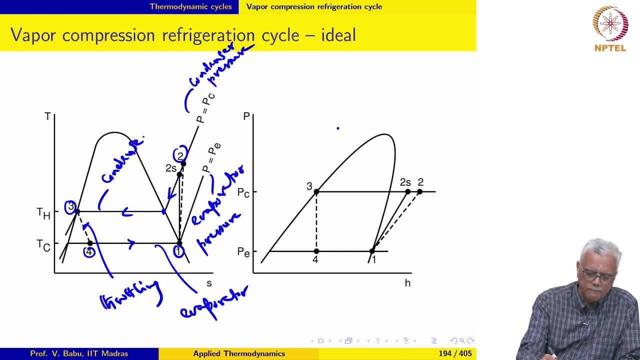 And this is the condenser. Okay, Now, this cycle is called the ideal vapor compression refrigeration cycle. Even if the compressor is not ideal, for example, even if the compression process has internal irreversibilities, this cycle is still usually referred to as the ideal vapor compression. 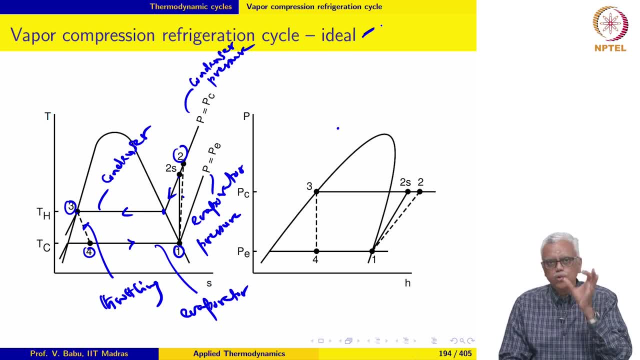 refrigeration cycle in the refrigeration community. There are two reasons for that. First one is that TH- Okay, TH is the temperature of the hot reservoir or the reservoir to which heat is rejected. So TH, usually in the case of an ideal vapor compression cycle, corresponds to the saturation. 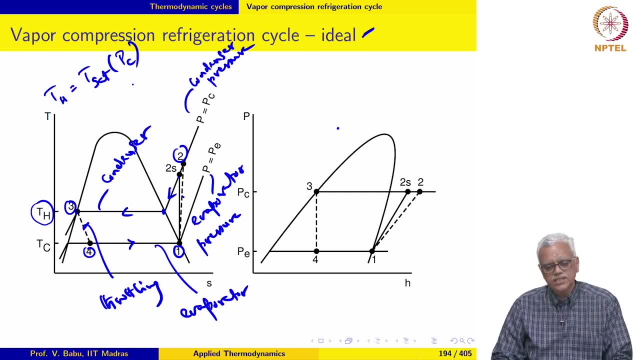 temperature of condenser pressure. Okay, So TH is TSAT of PC And TC, the temperature of the cold reservoir, or the cold reservoir from which heat is drawn by the refrigerant. Okay, Remember, TC is the temperature of the refrigerated compressor. 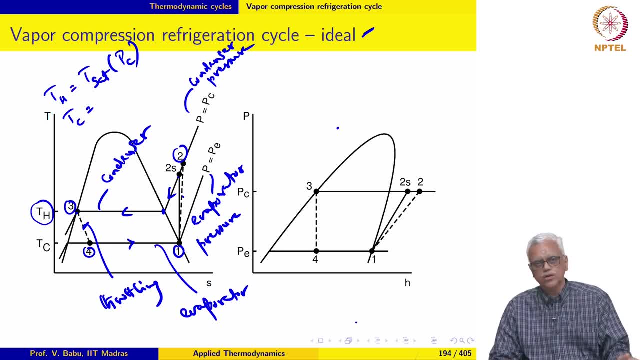 Okay, So this is where the heat is drawn by the refrigerant. So this corresponds to the saturation temperature of the evaporator pressure. Okay, That is number one. Number two, state one, is a saturated vapor in the case of the ideal vapor compression. 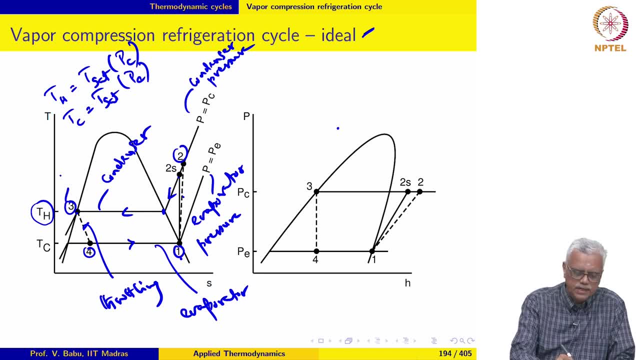 refrigeration cycle. And state three is a saturated liquid. So this is a saturated liquid and this is a saturated vapor. So TH is equal to TSAT of PC, TC equal to TSAT of PE. and state one: exit of evaporator is a saturated vapor state. exit of condenser is a saturated liquid state. 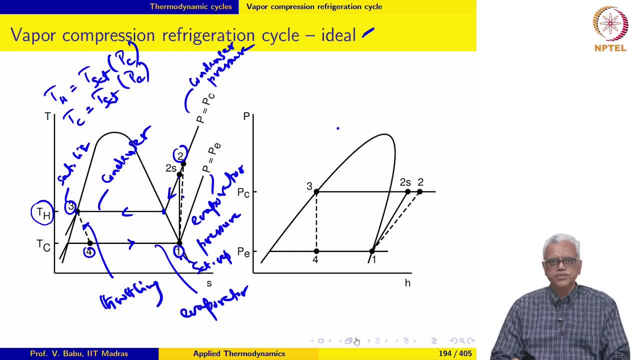 So this cycle is usually referred to as the ideal vapor compression refrigeration cycle in the refrigeration community. Okay, Now we may wonder, or you may wonder, why the diagram has to be illustrated in different, in a different set of coordinates. Why not just stay with TS? 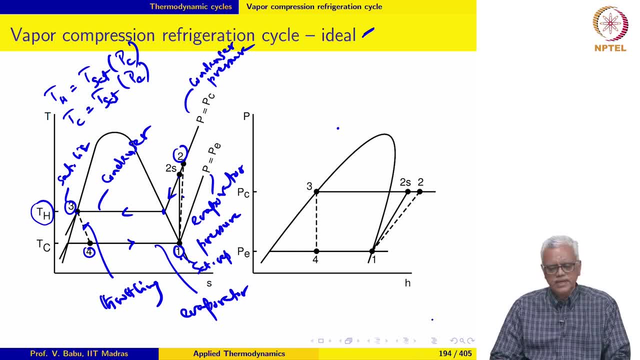 Why do we need this pH coordinates? Okay, It turns out to be an interesting question, So let us look at the processes that the refrigerant undergoes in the, in the, in the cycle. Okay, Okay, Okay, Okay Okay. 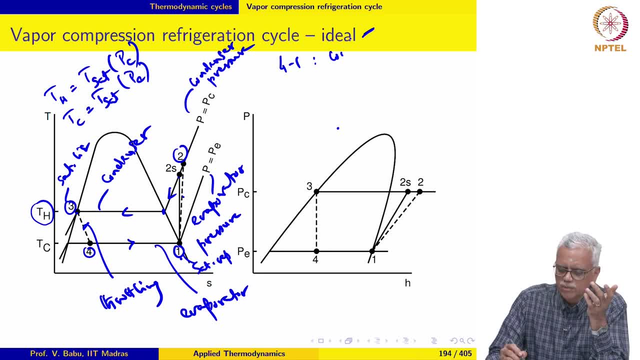 So phase change process and this, as you can imagine, is an isothermal process or isobaric process. Isobaric slash isothermal because it is a phase change process, That is, the process that the refrigerant undergoes in the evaporator. 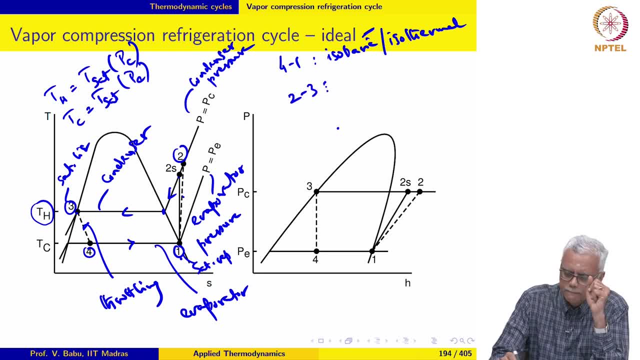 Okay Now 2, 3 is isobaric. Part of it is isothermal, But 2, 3 is isobaric. Okay, 2, 3 is isobaric. Pressure remains constant as the refrigerant loses heat to the ambient. 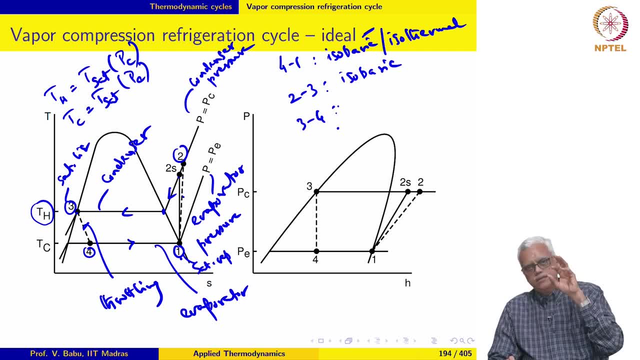 3, 4, assuming that the change in specific volume as a result of throttling is not very large, That the specific volume more or less remains the same. You know that throttling is an isenthalpic process, So this is an isenthalpic process. 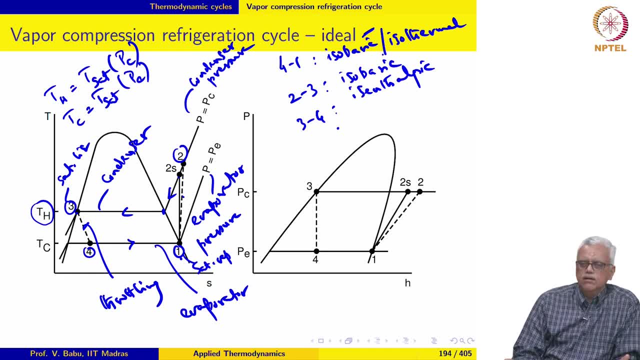 So you can see that 2 out of the 4 processes in the cycle- Okay, 1 process in the cycle or constant pressure processes, and 1 process is a constant enthalpic process. So which means if I choose P and H as coordinates, then the process will be straight line in. 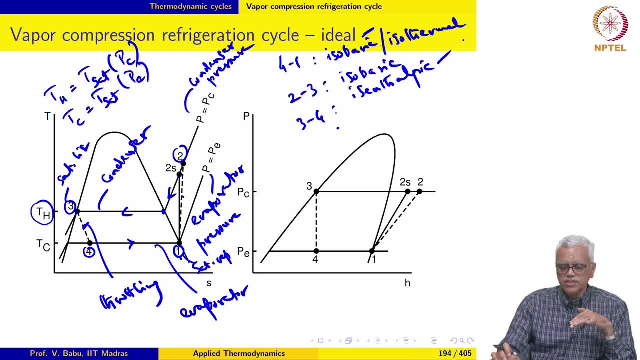 the in a P-H coordinate space and the third process, which is a throttling process, will also be a straight line aligned with the axis. Okay, So if I use P-H coordinates, then these 2 processes will be aligned with the coordinate axis. 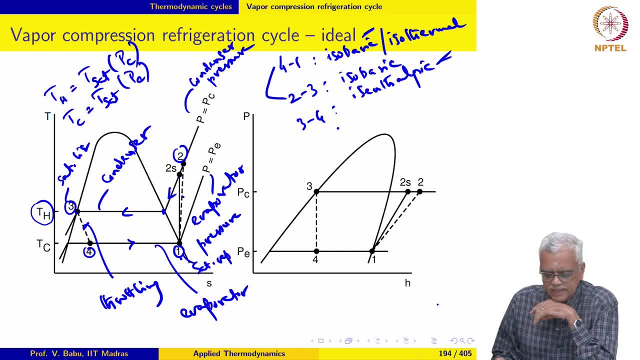 And this will be aligned with the other axis, which is why we would like to illustrate the vapor compression refrigeration cycle in a P-H diagram also, And this is extensively used in the refrigeration community. So, as you can see here, 4, 1 evaporator, constant pressure process at P-E, and 2S or 2 to 3 is. 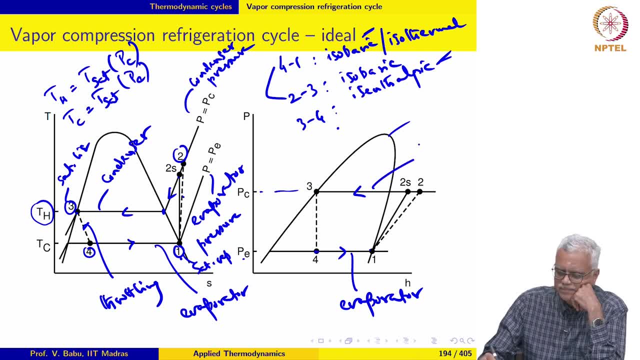 a constant pressure process at the condenser pressure: Okay. 3, 4 throttling process: constant enthalpy which is now aligned with the H equal to constant line. Okay, So 1 to 2S looks like this, in case the process actually has internal irreversibility still. 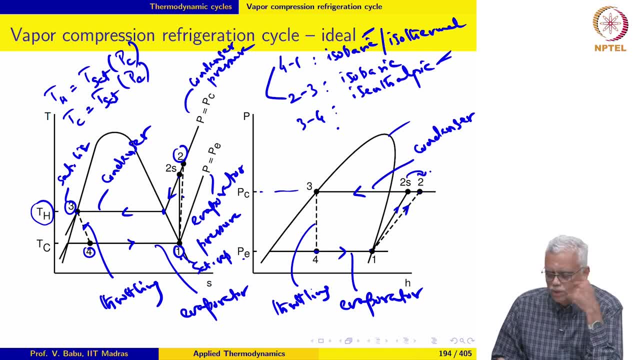 adiabatic. then the state point shifts from 2S to 2.. Okay, So the P-H coordinates actually are extremely just as useful as the T-S coordinates in depicting the process and is very widely used in the refrigeration community. 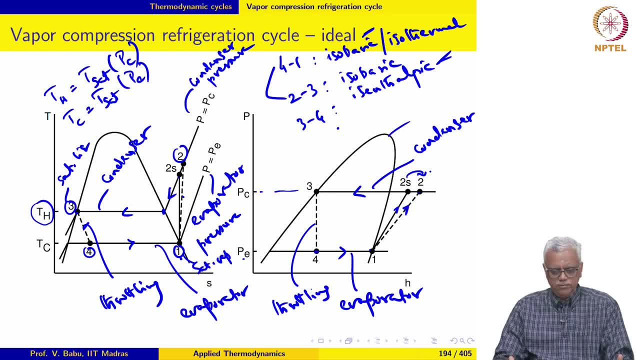 But in this course, though, we will stay with the T-S diagram. So this is an ideal vapor compression refrigeration cycle. Okay, So these points are very, very important. let me emphasize this again: T-H equal to T-SAT of P-C. 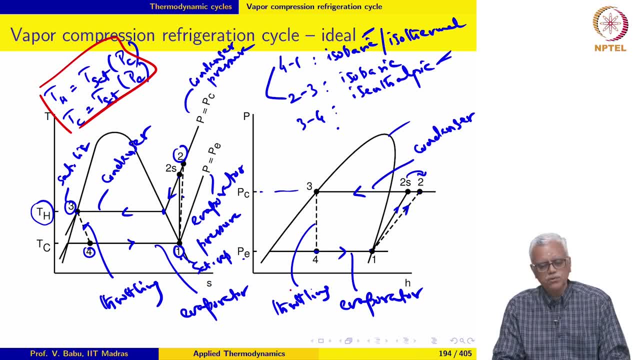 Okay, Okay, Pc. Tc equal to Tsat of Pe. So this is the Th is the temperature of the high temperature reservoir to which heat is rejected by the refrigerant. Tc is the temperature of the low temperature reservoir to which from which heat is absorbed by the refrigerant and saturated. 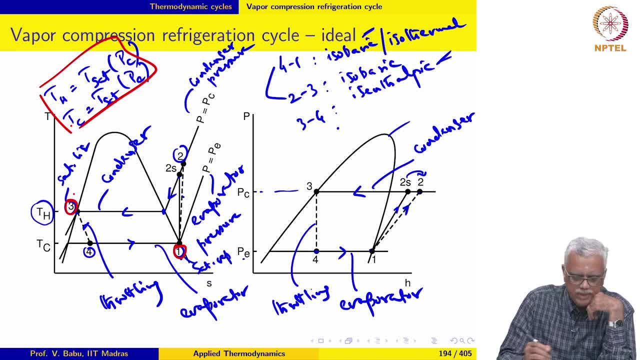 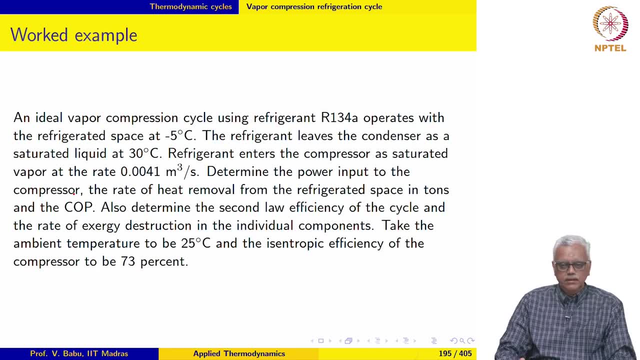 vapor at the exit of the evaporator. saturated liquid at the exit of the condenser. Let us go through a worked example now. So an ideal vapor compression cycle using refrigerant R134a. we no longer use R134a because it is not environmentally friendly. we have much. 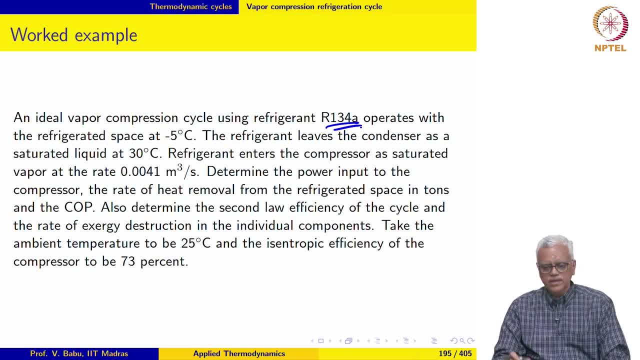 better refrigerants now. But we use R134a in the core For purposes of illustration only. this can be replaced with any other refrigerant once the property values, the property tables, are available. So here it is, given that this is an ideal. vapor compression, refrigeration cycle Temperature. 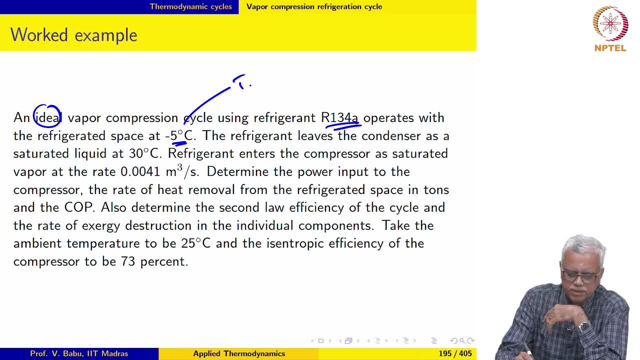 of the refrigerator space is minus 5 degree Celsius, So that means Tc is equal to minus 5 degree Celsius. The refrigerant leaves the condenser as a saturated liquid at 30 degrees Celsius, So that means TH is equal to 30 degree Celsius. 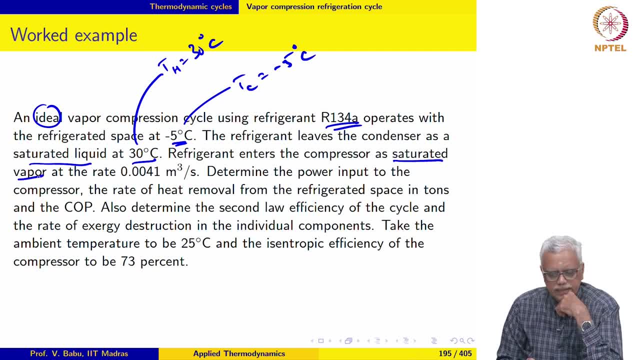 Refrigerant enters the compressor as saturated vapor at the rate of 0.0041 meter cube per second, whereas to determine the power input, rate of heat removal and COP, as well as the second law efficiency and rate of exergy destruction in the individual components. 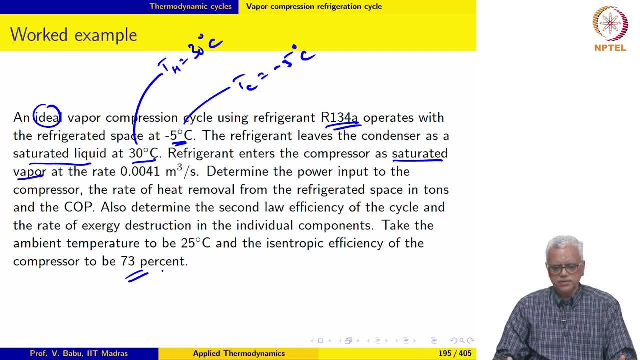 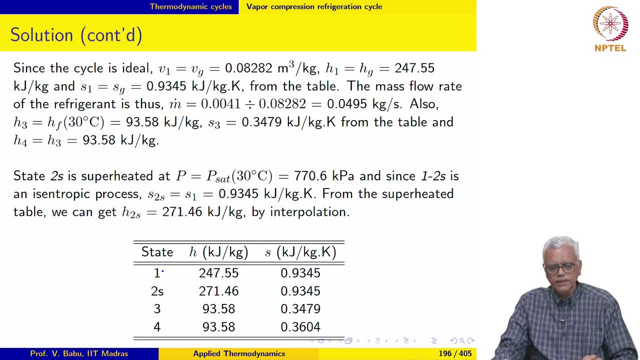 The isentropic efficiency of the compressor is given to be 73 percent. So this is an ideal vapor compression cycle. Since it is ideal state, point 1 is a saturated vapor at entry to the compressor. So V1 equal to Vg and H1 equal to Hg and S1 equal to Sg from the saturated temperature. 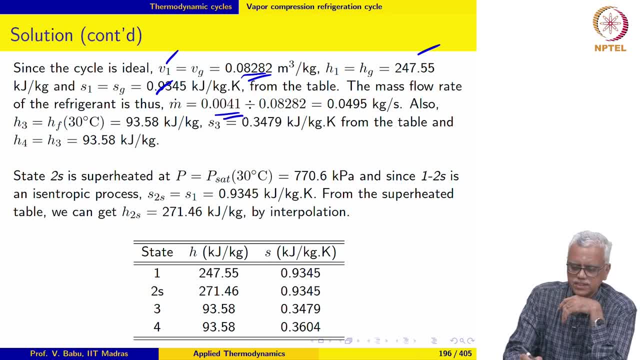 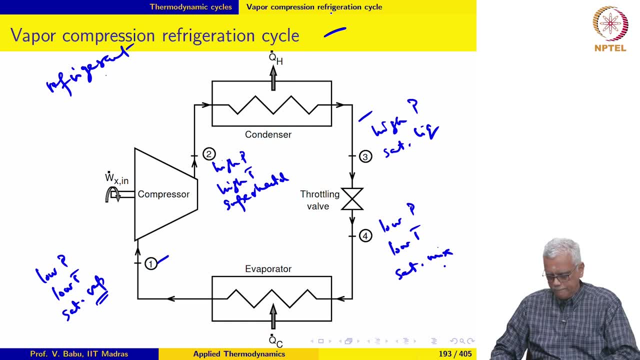 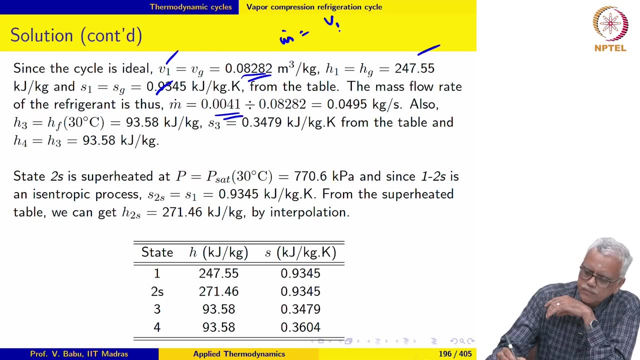 table. So the mass flow rate of the refrigerator is given to be 73 percent. Since volume flow rate is given, m dot is equal to V1 dot, the volume flow rate. Since volume flow rate is given, we may evaluate m dot equal to V1, dot over V1, and that is. 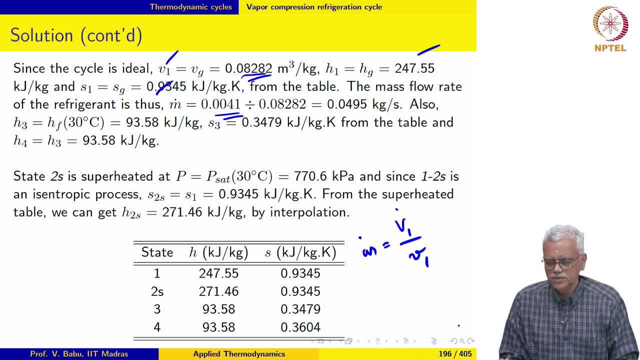 what we have done here. So that is it. So the mass flow rate comes out to be 0.0495 kg per second. H3 is equal to Hf at 30 degree Celsius, because it is an ideal vapor compression cycle. S3 may also be retrieved from the table. 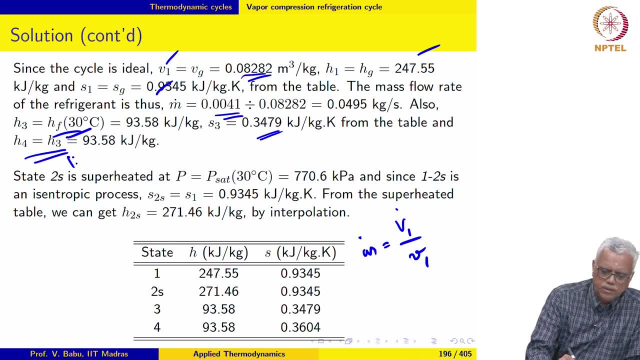 and H4 equal to H3 because throttling is an isentropic process, so H4 equal to H3.. State 2s is superheated at a pressure which is Psat of 30 degree Celsius, So that pressure corresponds to 770.6 kilo Pascal. 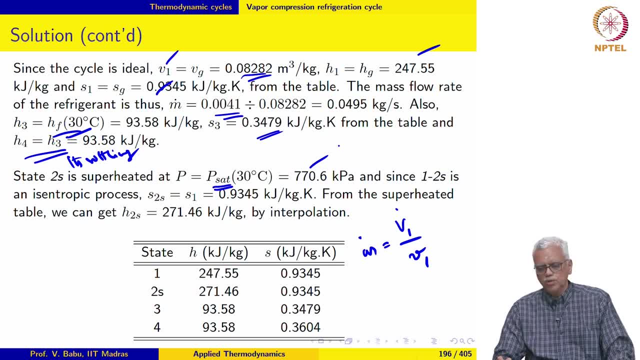 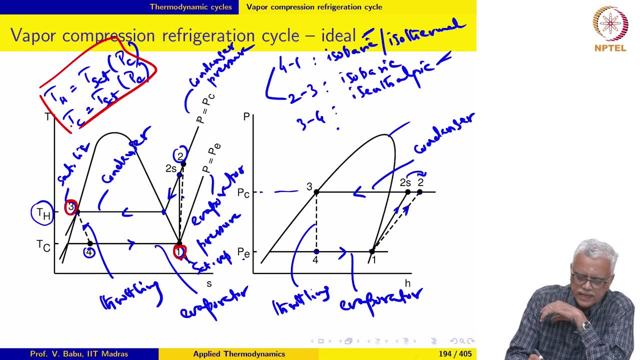 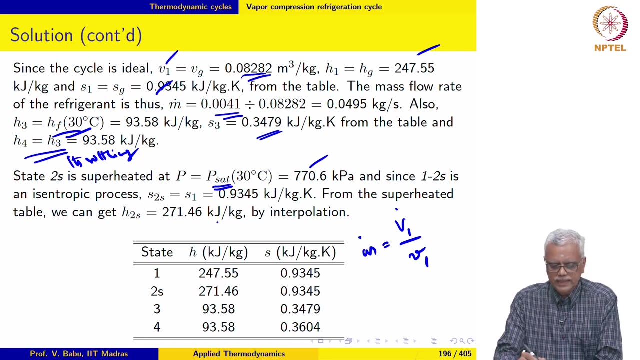 Let us just take a quick look here. So state 2s is a superheated state at a pressure Pc which corresponds to the saturation pressure of Th or 30 degree Celsius. So we can get H2s from the superheated table through interpolation. 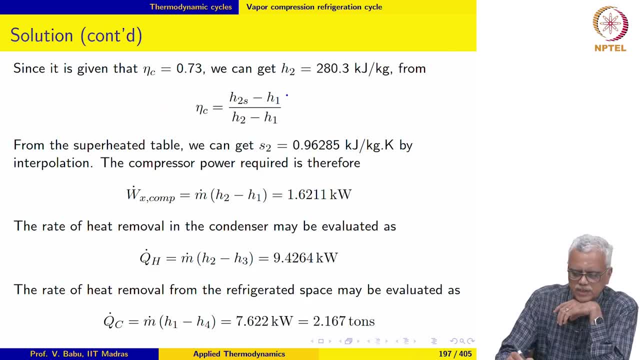 And the isentropic effect is the same. So we can get H2s from the superheated table through interpolation. So we can get H2s from the superheated table through interpolation. So the isentropic efficiency of the compressor is given to be 73 percent. 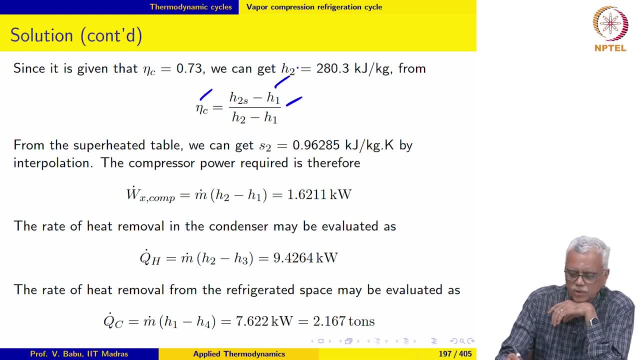 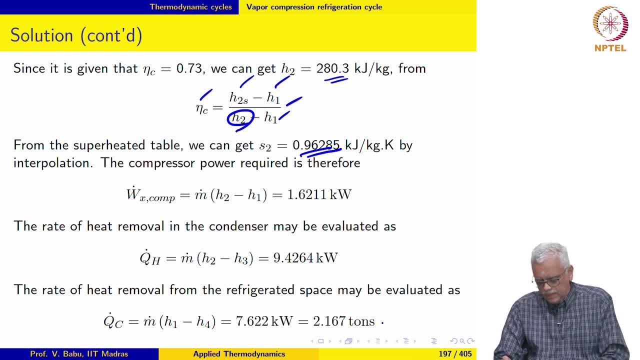 S2 to be 0.96285.. What is that? This is more than the value for S2s, S2S. S2S is 0.9345.. So S2 is equal to 0.96.. So the state at the exit of the compressor. 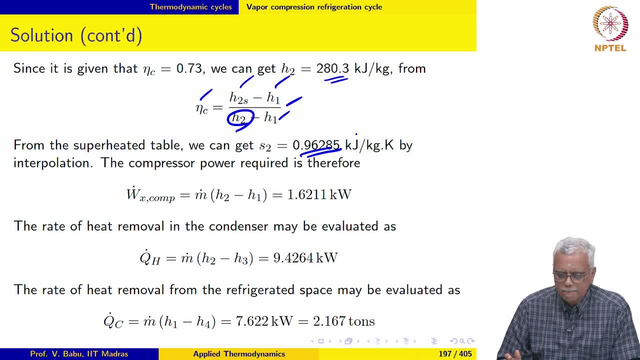 lies to the right of state 2S. So from steady flow energy equation we may get the compressor power to be 1.6211 kilowatts. And again from steady flow equation applied to the condenser we can get the heat removed in the condenser to be 9.4264 kilowatts. And by applying steady 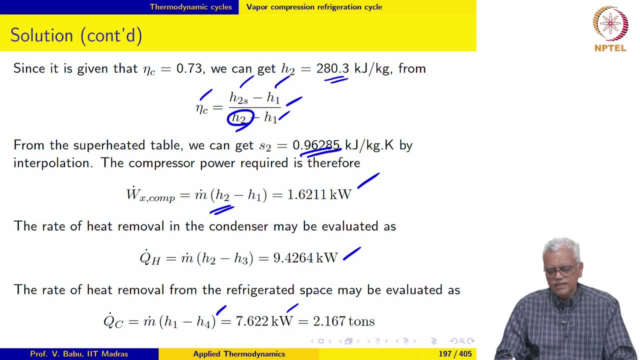 flow energy equation to the evaporator. we may get the heat removed in the evaporator to be 7.622 kilowatts, but we have been asked to evaluate this in tons. So 1 ton of refrigerator- refrigeration, I am sorry- is equal to 211 kilo joule per minute. a heat removal rate. 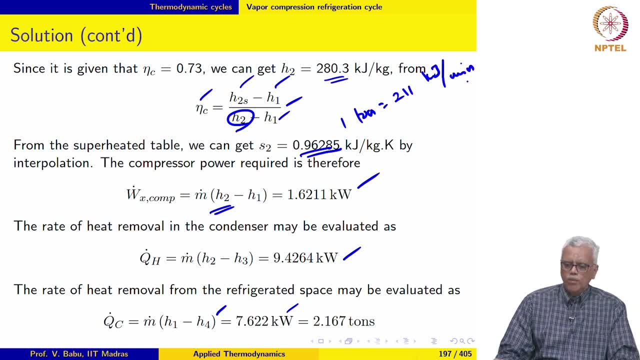 of 211 kilo joule per minute. So 1 ton of refrigeration is defined as the heat removal rate that is required to convert 1 ton of water- liquid water at 0 degree Celsius to ice at 0 degree Celsius in 24 hours. That is the definition for 1 ton of refrigeration and that corresponds. 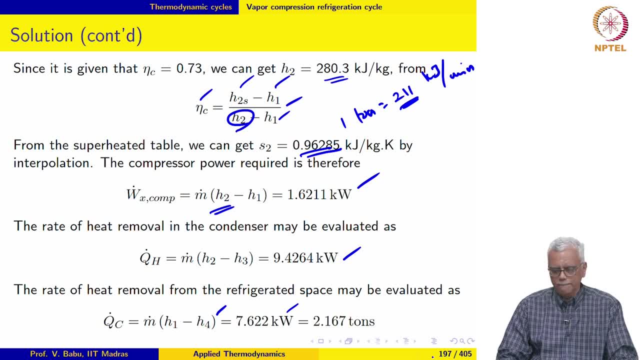 to a heat removal rate of 211 kilo joule per minute. So we may then convert 7.622 kilowatts to 2.167 tons. So you may recall that when you go to the shop to buy an air conditioner, for instance, 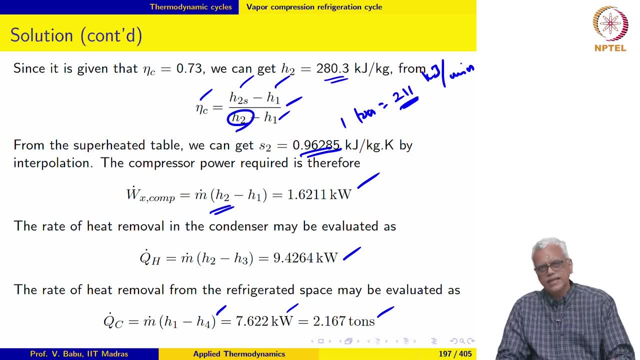 you are normally asked, I know, do you want a 1 ton AC, 2 ton AC and so on. So that is what the ton, the terminology, that is, this is what it means. So COP for the refrigerator. 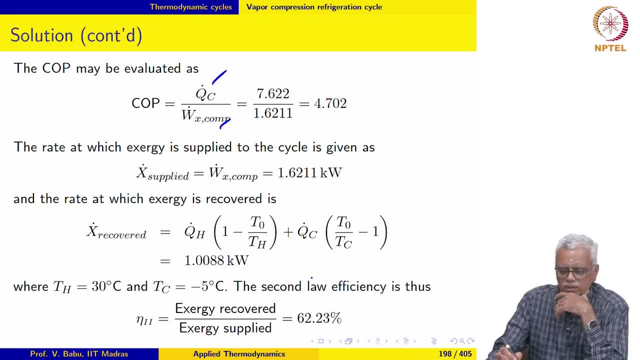 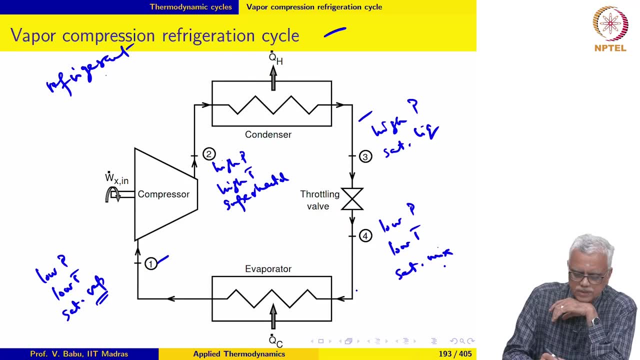 is nothing but QC dot divided by power input to the compressor and that works out to 4.702.. Now if you go back to the cycle, notice that XRG is required and in the condenser XRG is recovered, and in the evaporator also. 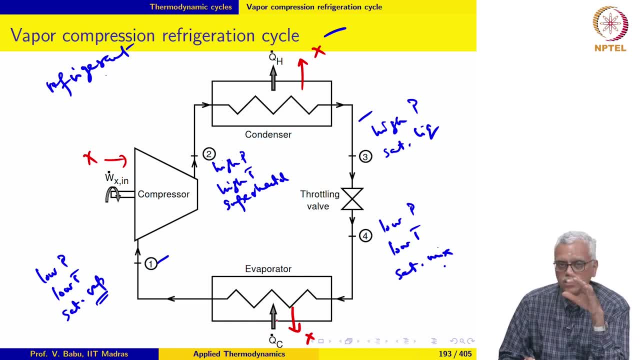 XRG is recovered. Please go back and check the module on XRG. this is the low-temperature reservoir, which is actually from which heat is extracted. So that means XRG is recovered. In this case the sine for X and Q are opposites, so here X is supplied and X is required in. 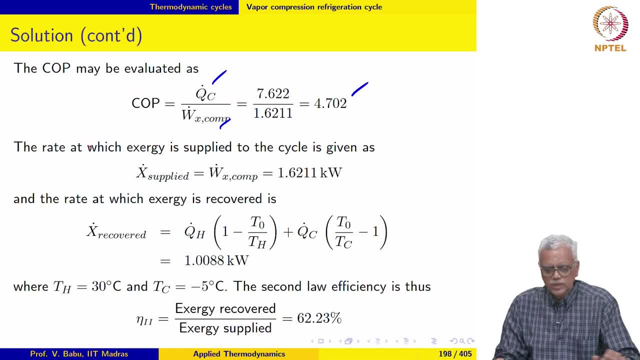 these two devices, So x applied is equal to the power, So x dot recovered is what we get in the condenser where heat is rejected. So here the direction of heat flow and the direction of exergy flow are the same, whereas here the direction of heat flow and direction of exergy flow are. 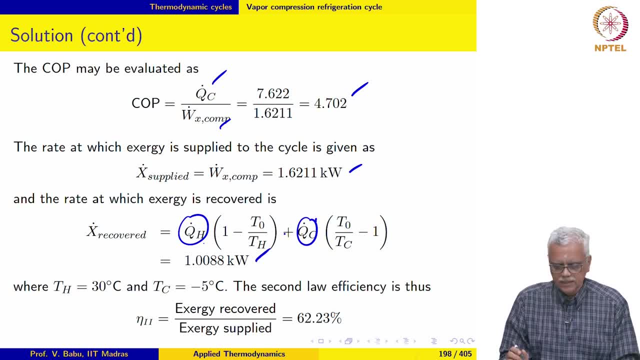 opposite. So this is x. recovered, that comes out to be 1.0088 kilowatts. Notice that T H in this case is 30 degree Celsius. that is a temperature of the reservoir to which heat is rejected by the refrigerant. This is the temperature of the reservoir from which heat 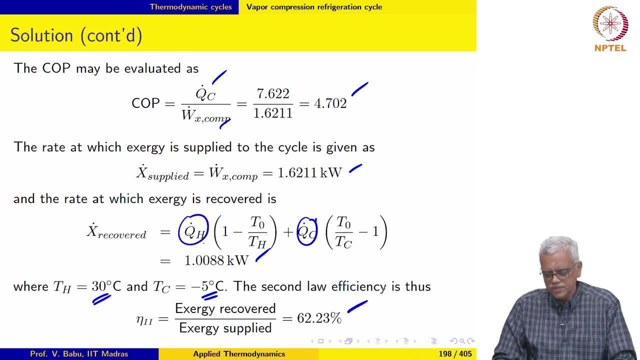 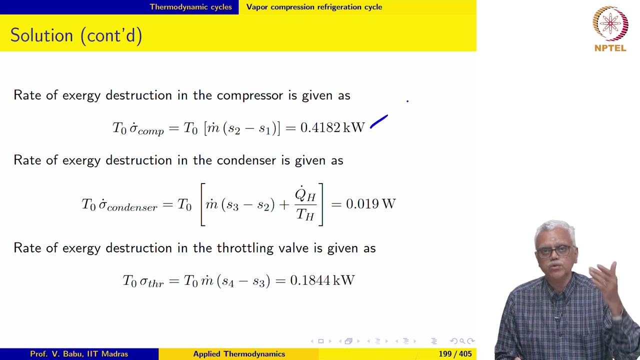 is extracted by the refrigerant. So the second law efficiency comes out to be 62.23 percent. So this aspect is very important. So you must bear this in mind, that this is exergy that is recovered. Now if we apply entropy balance equation to the individual components, 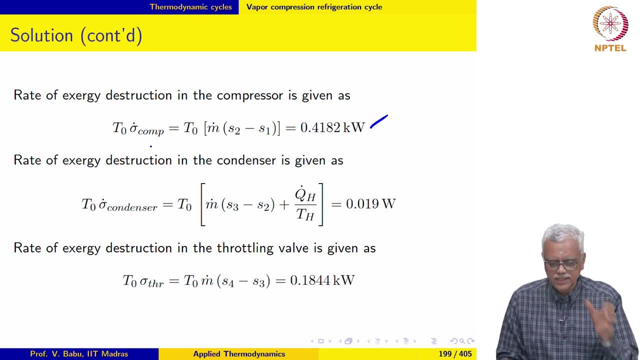 we can see that the temperature of the reservoir is equal to the temperature of exergy flow. So we can get the following things. So rate of exergy destruction in the compressor works out to 0.4182.. There is no heat loss from the compressor because it is still adiabatic. 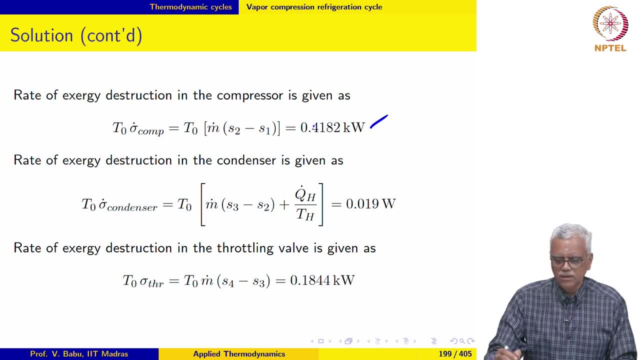 although internally irreversible. So this loss of exergy or entropy generation is due to internal irreversibility in the compressor, No external irreversibility because it is insulated. Rate of exergy destruction in the condenser: again this is 0.4182.. So this 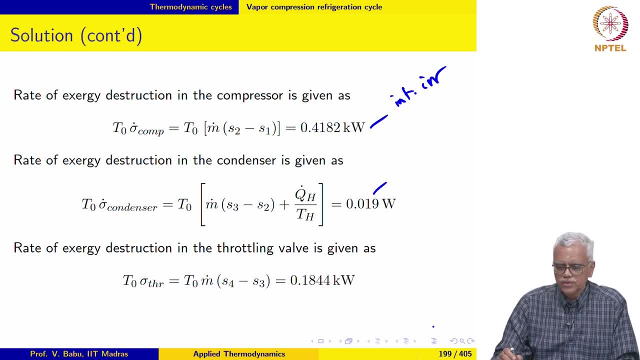 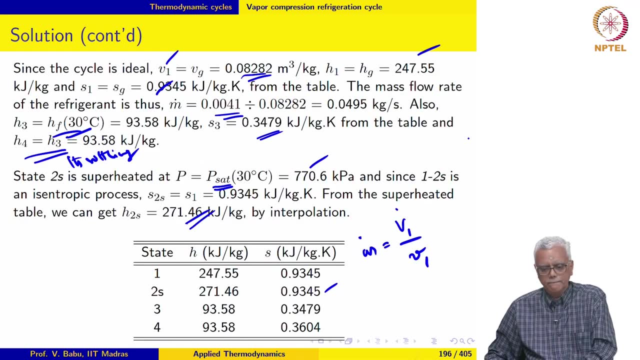 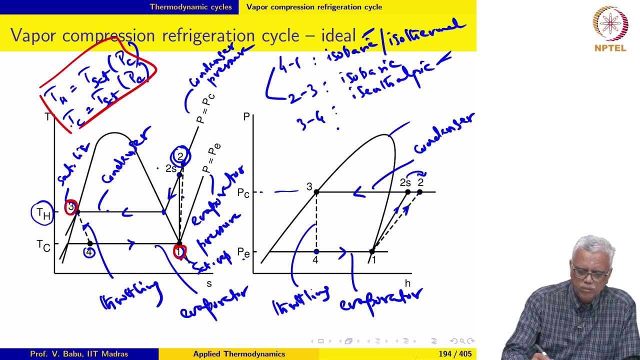 is heat transfer across a finite temperature difference. So this is due to external irreversibility. So you may see that when the refrigerant enters the condenser it is at a much higher temperature compared to TH. So there is heat loss across a finite temperature difference. 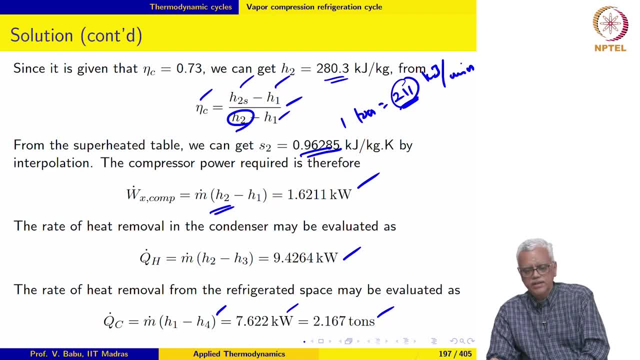 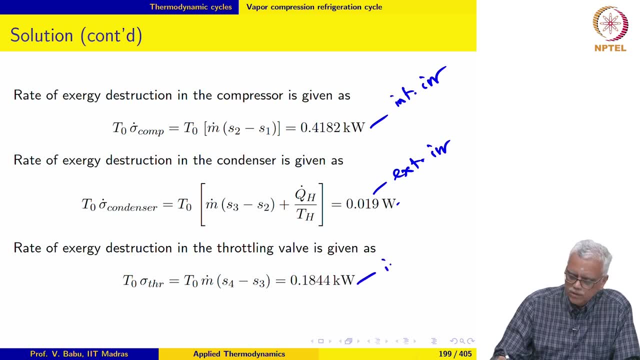 which is why we have entropy generation or exergy destruction in the compressor. So this is due to internal irreversibility in the condenser. Throttling, as we already saw, is an internally irreversible process, So the exergy destruction is due to internal irreversibility. But if you look at the exergy destruction in the 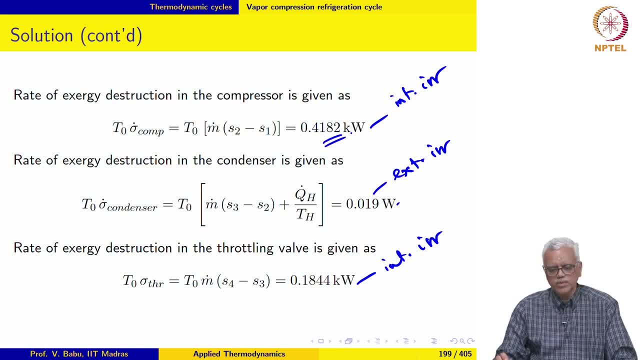 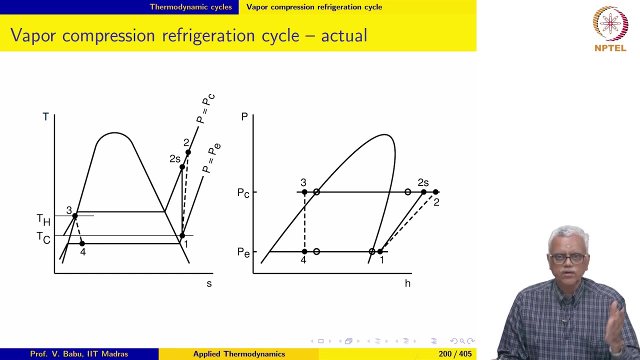 components. you can see that the maximum contribution comes from the compressor. others contribute quite less than what we get from the internal due to internal irreversibility in the compressor. So this is what we get Now. we have looked at the ideal vapor compression refrigeration cycle In the case of an actual 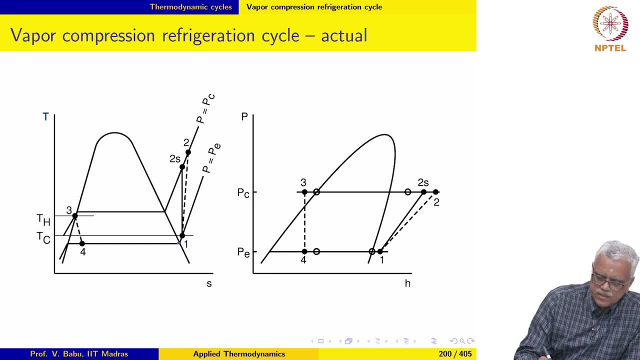 cycle. it can never be guaranteed that the state at the exit of the evaporator will always be a saturated vapor. In general, the state at the exit of the evaporator is slightly superheated. Similarly, we can never always guarantee that the state at the exit of the condenser will. 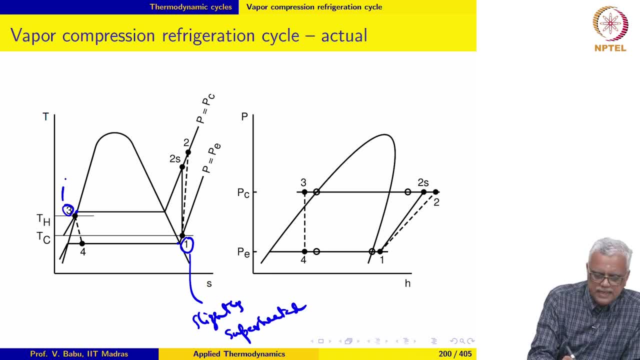 be a saturated liquid. it is almost always slightly compressed, or we may say this is a compressed liquid state And notice in this case that TH is not the same as T sat of Pc. TC is not the same as a T sat of Pe. 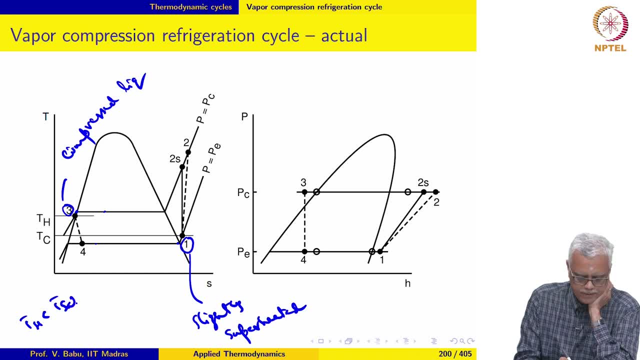 So TH in this case is less than T sat of Pc And TC is equal to T sat of Me. So it is the same SH. TH, Pc and TC are the same is, I am sorry, greater than T sat of P? e. Now T c has to be greater than T sat of P. 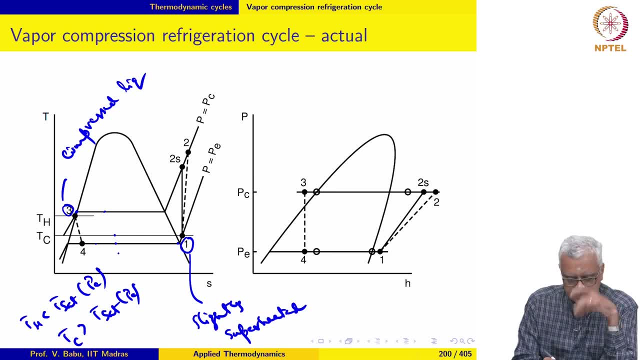 e, because that is the only way heat can be extracted by the refrigerant from the refrigerated space. Similarly, T h has to be less than T sat of P c, because that is the only way heat can be transferred from the refrigerant to the ambient or high temperature reservoir. 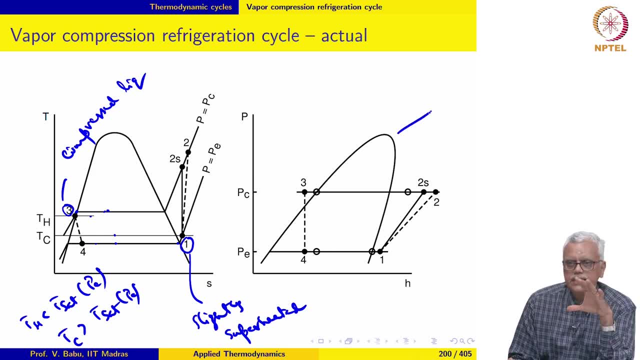 So we see here the actual cycle illustrated on a pH diagram. The open circles indicate the ideal vapor compression cycle and the actual compression cycle. as you can see, here it is slightly superheated and here it is slightly subcooled, and that may be a better. 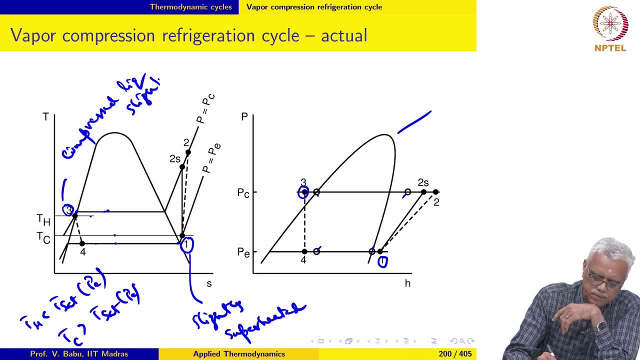 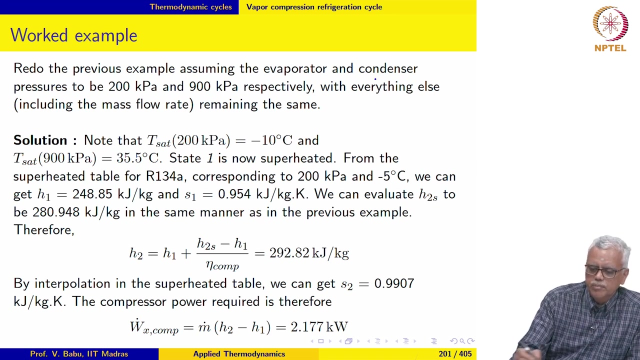 terminology, So compressed liquid or slightly subcooled. Okay, Now let us see what changes in the performance matrix this makes in going from ideal cycle to the actual cycle. So we will redo the previous example. but now we take the evaporator. 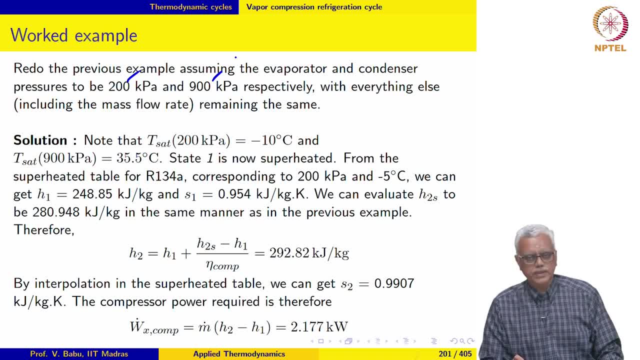 and condenser pressure to be 200 and 900 kilohertz- Okay, 900 kilo Pascal- respectively. So this means that T h remains at 30 degree Celsius and T c remains at minus 5 degree Celsius, But we have changed the evaporator and the condenser. 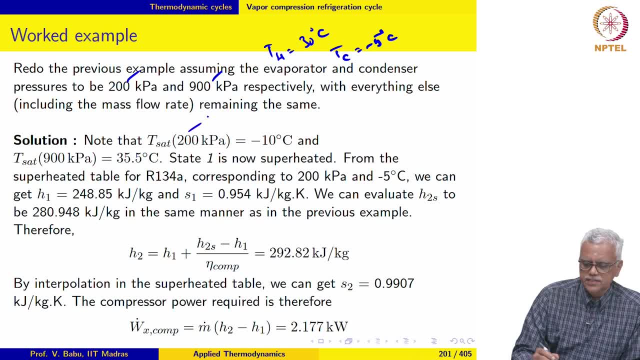 pressure. So, interestingly, you can see that T sat, corresponding to the evaporator pressure, is minus 10 degree Celsius. Okay, So you can see that T c is greater than T sat corresponding to T e. Okay, So then heat. 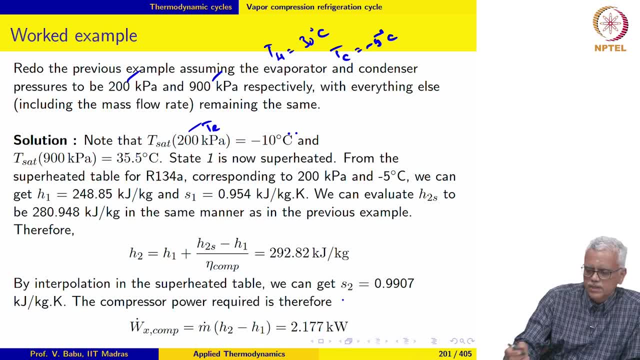 can be abstracted by the refrigerant from the refrigerator compartment. So refrigerator compartment is maintained at minus 5 degree Celsius, but the refrigerant is at a temperature of minus 10 degree Celsius when it enters the evaporator. So that means heat flows. 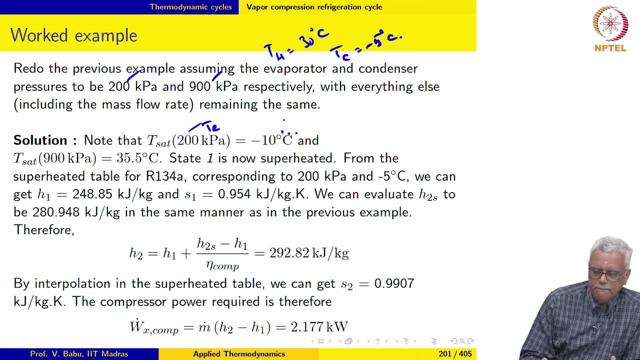 from the refrigerator compartment to the refrigerant. Okay, Okay, Okay, Okay Okay. Similarly, T sat, corresponding to the condenser pressure, is 35.5 degree Celsius, whereas the ambient temperature is 30 degree Celsius, So heat transfer can comfortably take place. 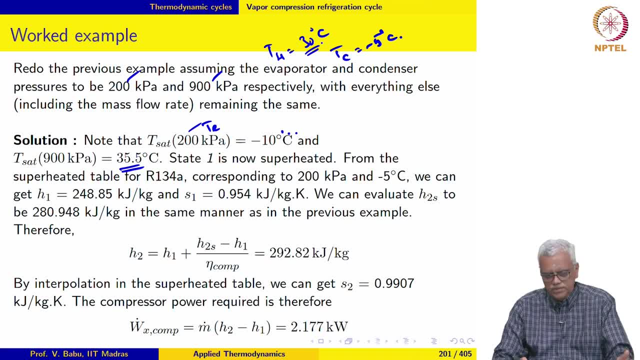 between the refrigerant and the ambient. So state 1 now is slightly superheated. So from the superheated table we can retrieve appropriate property values H1 and S1.. Okay, Okay, Okay, Okay, Okay. 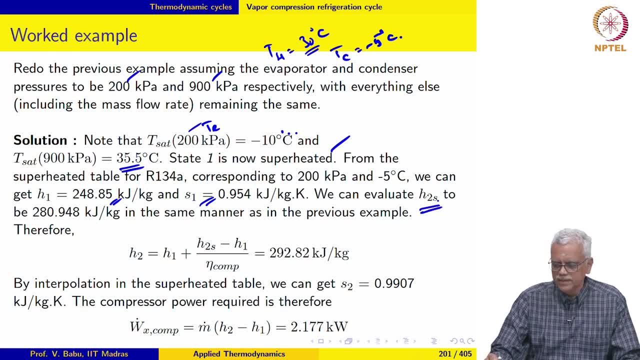 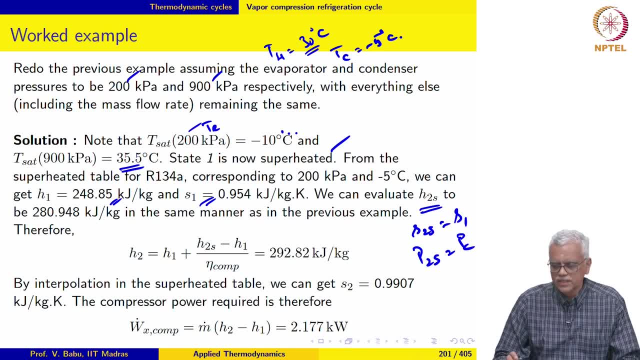 S1 and P2S equal to Pc, the condenser pressure. So once we do that, we can evaluate H2, or yes, we can evaluate H2 by making use of the definition of the isentropic efficiency of the compressor, and H2 comes out to be 292.82 kilo joule per liter. 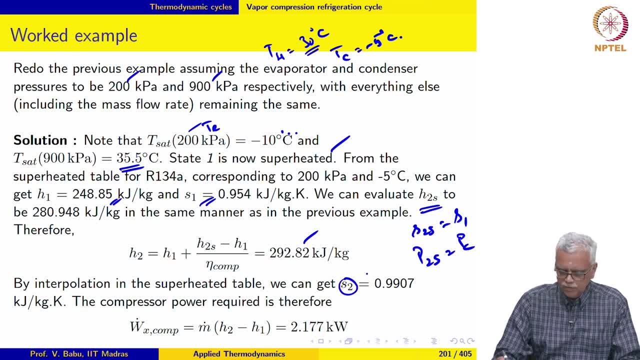 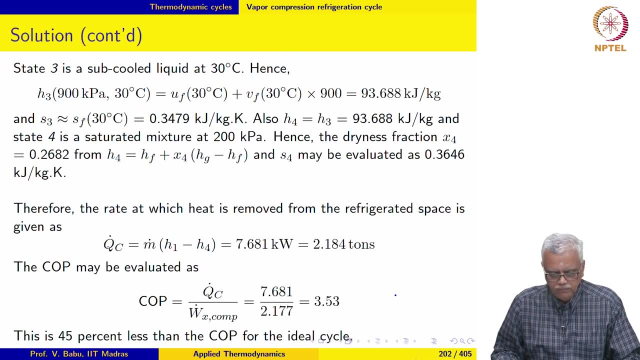 kilogram And the corresponding value for specific entropy may be evaluated by interpolation from the superheated table. So the power required now comes out to be 2.177 kilowatts. Now, state 3 is a subcooled liquid. Notice that state 3, at state 3, the pressure of 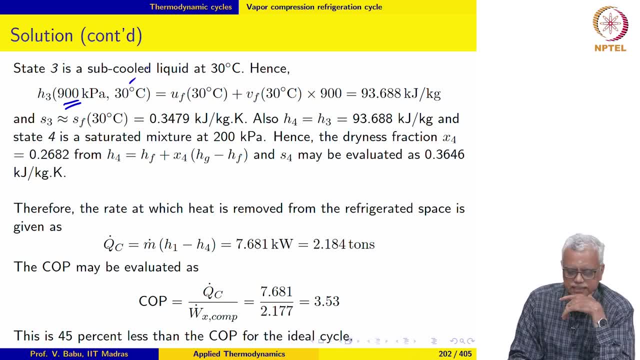 the refrigerant is 900 kilo Pascal, temperature is 30 degree Celsius, So it is a compressed liquid or subcooled liquid, and we evaluate the enthalpy using this approximation. So this is actually an approximation and the specific enthalpy comes out to be 93.688, and 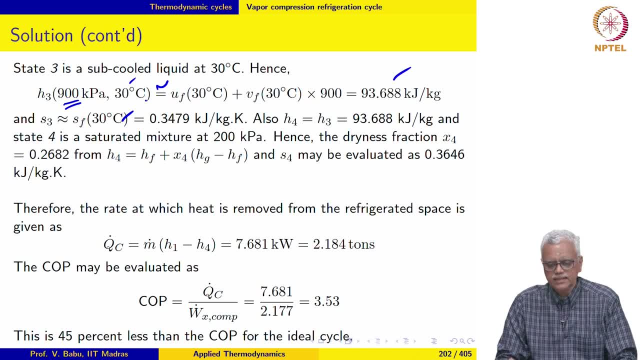 S3 comes out to be equal to Sf, approximately at 30 degree Celsius. Now H4 equal to H3 still, Because it is an isenthalpic process and dryness fraction at state 4 may be evaluated from here and using this dryness fraction, S4 may be evaluated just like what we did. 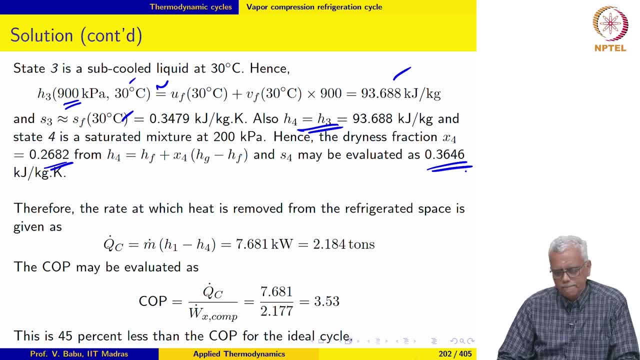 before as 0.3646.. So notice that from state 3 to state 4, the specific entropy increases, as it should, because throttling is an isenthalpic process. So these are consistency checks that you can use When you are doing the calculation. just make sure that the numbers that you are getting 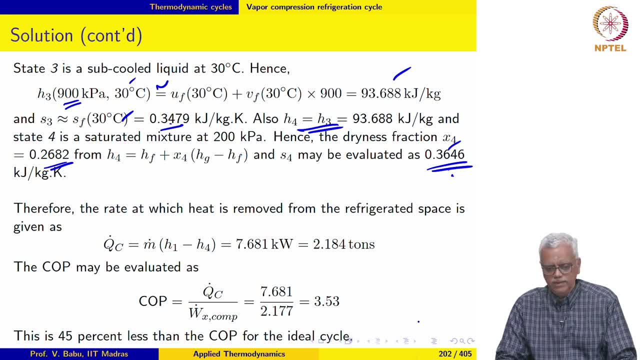 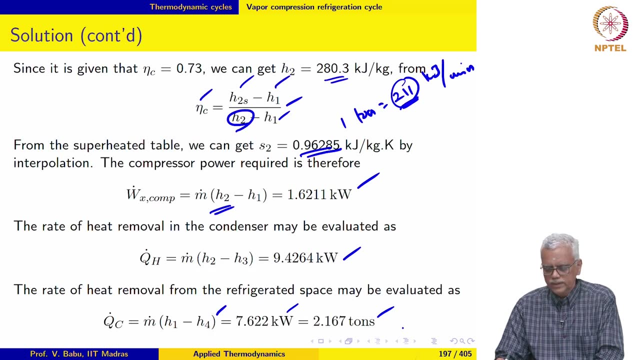 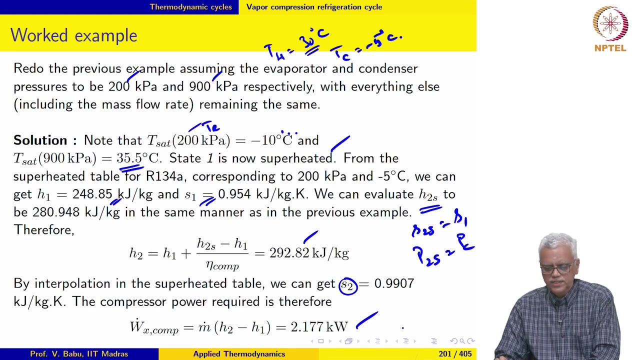 are what they ought to be, at least qualitatively. So rate of heat removal from the refrigerator space is 2.184 tons compared to 2.167 tons. So more heat is removed now. Mass flow rate of the refrigerant remains the same. 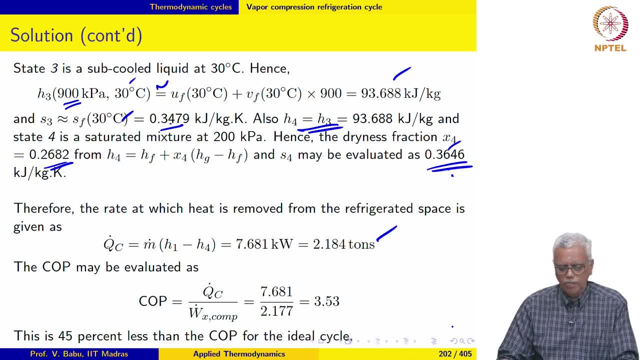 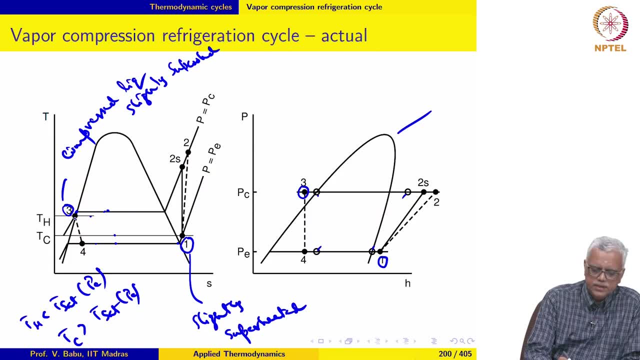 So the reason for this is that state point 3 has now moved to the left of where it was before, which means that state point 4 is going to be further to the left of where it was before. This is very evident here, so which means if it is over here, then the amount of heat. 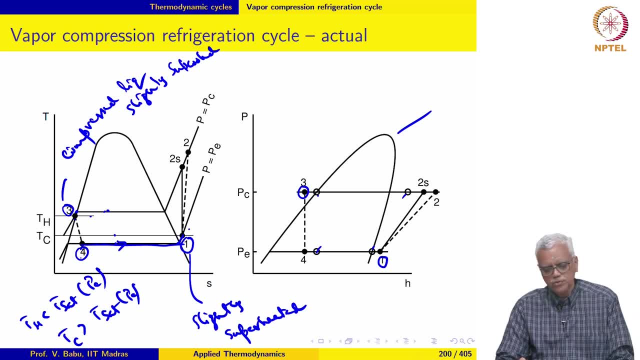 that can be removed from the new state point 4 to the new state 1 is going to be more than what it was before. So earlier state point 4 was over here and state point 1 was over here. So the amount of heat that could be removed earlier was less than what it is now. 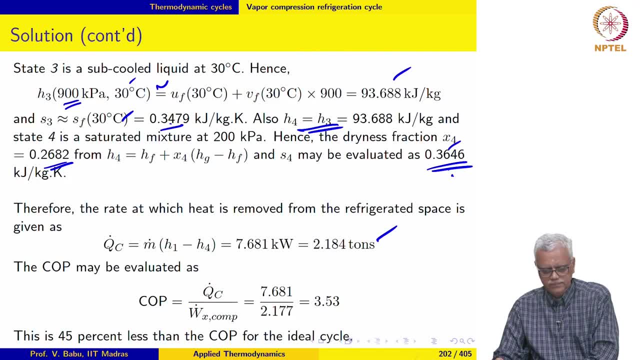 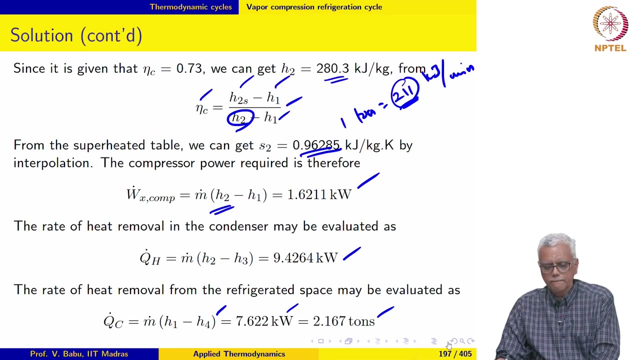 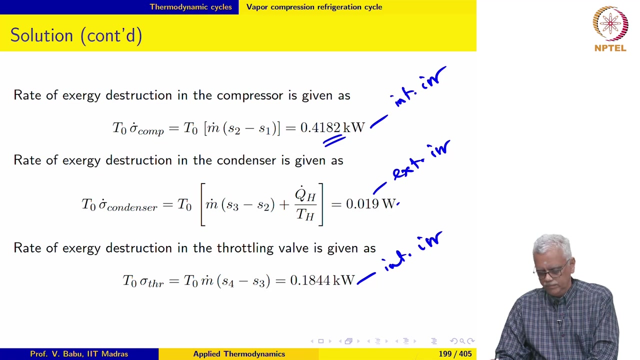 So the COP for the cycle comes out to be 3.53, which is less than what we had before. The heat removal has increased, However, the power has also. if you look at the power, this is 2.177 and earlier we had 1.6211 kilowatts. 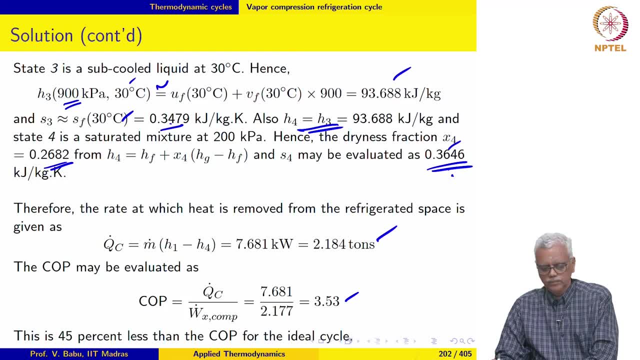 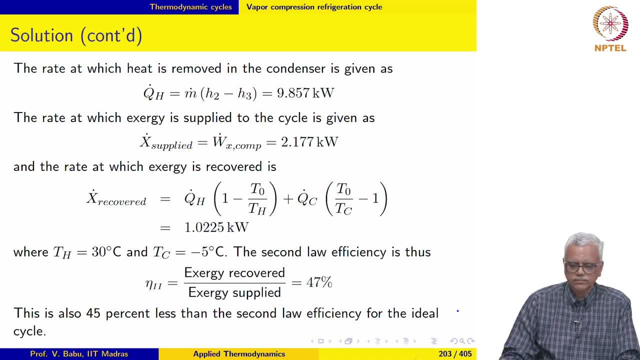 This is 45 percent less than the COP for the ideal cycle. Okay, So rate of heat removal in the condenser: again from steady flow energy equation comes out to be 9.857.. And once again, exergy supplied in the cycle is equal to the power that is given to the 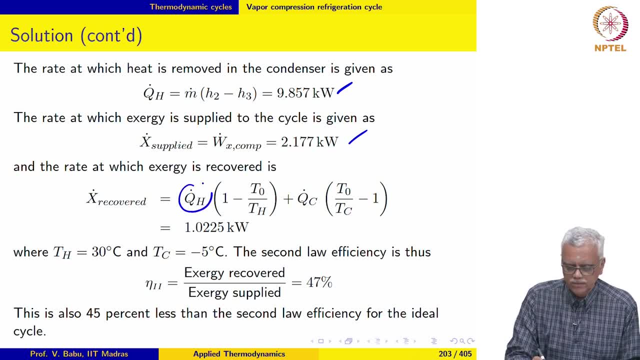 compressor, So that is 2.177, and exergy recovered from the condenser and from the evaporator. So together it comes out to be like this: Notice that T h is still 30 degrees Celsius, T c is still minus 5 degrees Celsius, as we 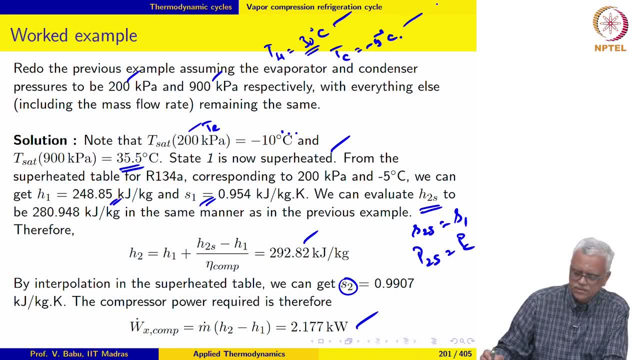 wrote down here. Okay, So T h is still 30. This is still minus 5.. I am sorry, So the second law efficiency comes out to be 47 percent only, which is actually 45 percent less than the second law efficiency for the ideal cycle. 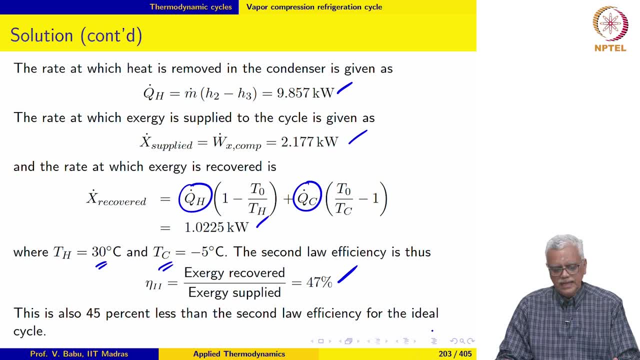 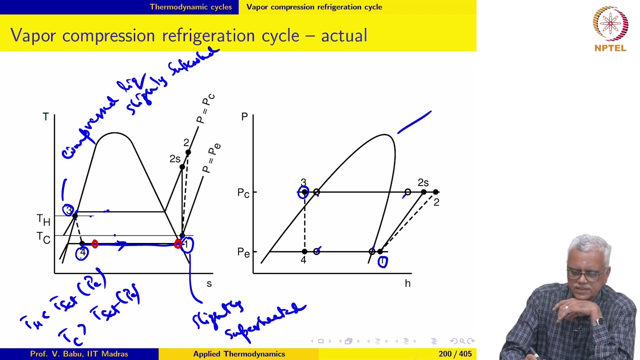 Again, this is due to the fact that this is due to the fact that the, if you look at the cycle, You can see that now the temperature differences, in this case, or external irreversibility, increases in the condenser, So the loss of or the destruction of exergy is going to be higher in the condenser. 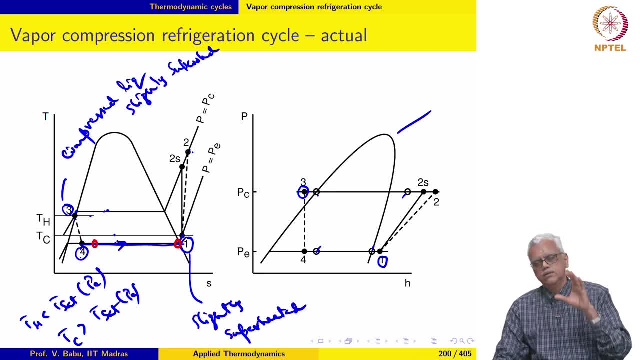 So earlier all the exergy destruction was in the compressor. Now the exergy destruction in the compressor more or less remains the same, But the exergy destruction in the condenser has increased considerably and the exergy destruction in the throttling valve also increases somewhat because of the fact that it is now 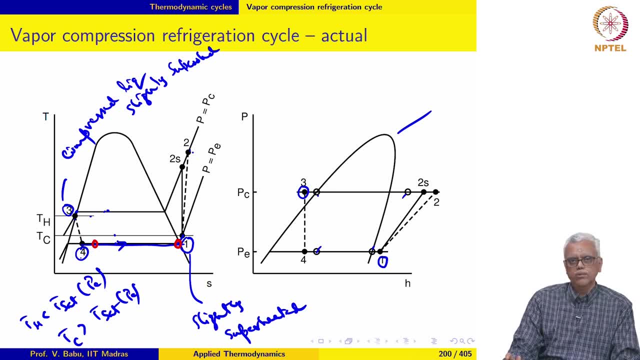 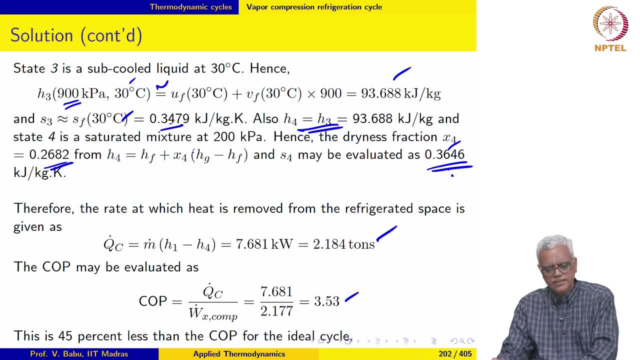 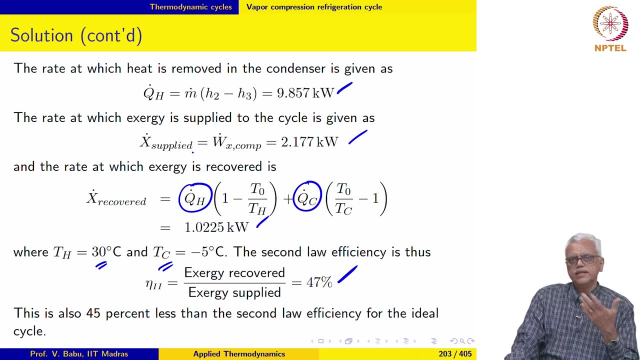 entering as a slightly sub-cooled liquid Because, as I said before, the vapor compression refrigeration cycle is used mostly in domestic applications: refrigerated air conditioners. It can also be used in for cooling of buildings and so on. But a single refrigerate, single cycle or a cycle with a single refrigerant will not. 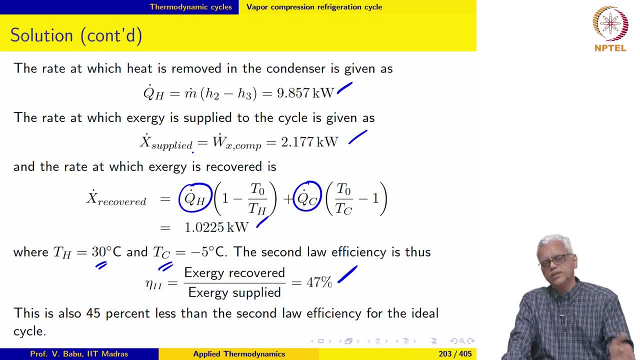 be adequate for such purposes. So normally you either use a cascade refrigeration system which cascades one refrigerant cycle on top of the other. So that is one way of doing this, Because there are also there is also something called a multistage refrigeration cycle, which 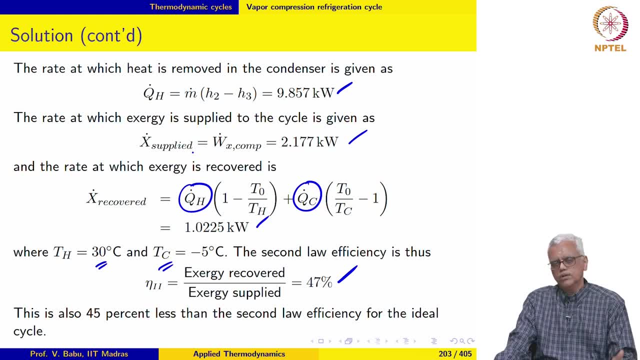 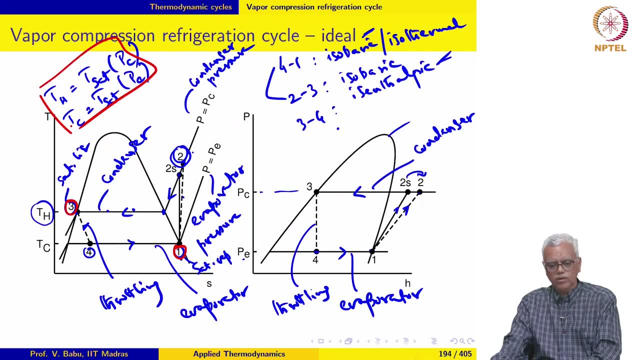 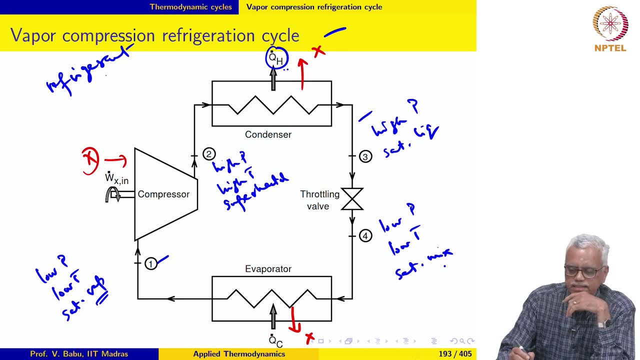 uses multiple stages to do this. Both are acceptable. Basically, the idea is so. if you go back to the block diagram, the basic idea is this: heat rejection. in the case of a multistage or cascade sort of cycle, this heat rejection does not take place to the ambient, but it actually this condenser for one cycle becomes. 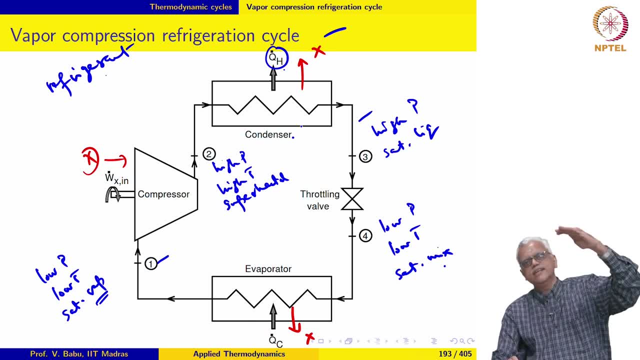 a evaporator for the next cycle And that the condenser for the second cycle, which is the outflow. So this is the evaporator for the next cycle And that the condenser for the second cycle, which is the outflow, which is the outflow. 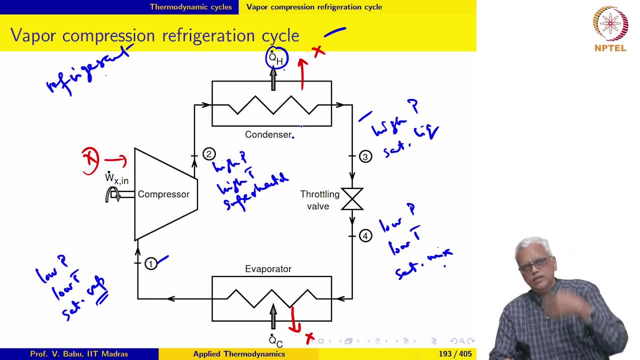 for the upper cycle will then reject heat to the ambient. So that is how these are coupled, and together this can give very good performance and can be used for even larger applications than the refrigerator or air conditioner. Of course, one important aspect about the vapor compression refrigeration cycle and 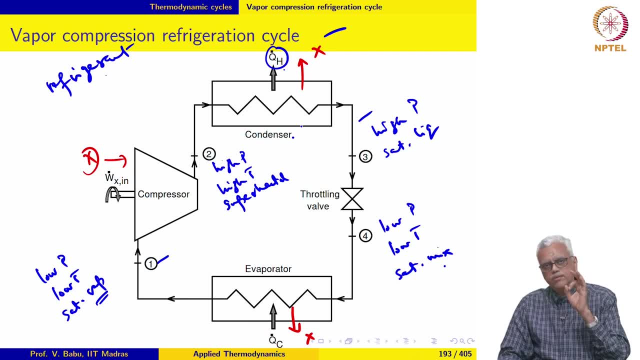 indeed, refrigeration is the use of environmentally friendly refrigerants. We have not paid any attention to that. When you do a course on refrigeration and air conditioning, the details and the impact of refrigerants on the environment will be discussed in great, in great length. 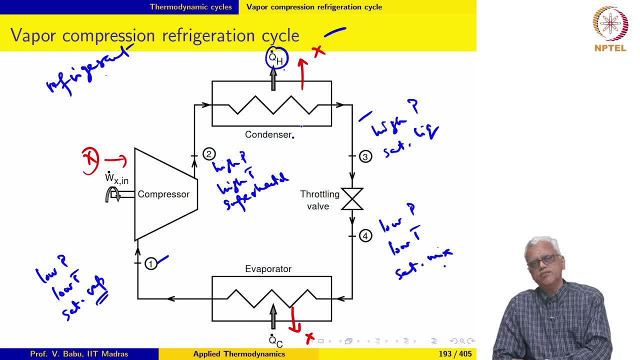 This is very important because the refrigerants have the potential to cause damage to the ozone layer and also cause global warming. So we need environmentally friendly refrigerants, which is what we are using nowadays, Plus other refrigerants which are nonflammable, which have much better environment friendly. 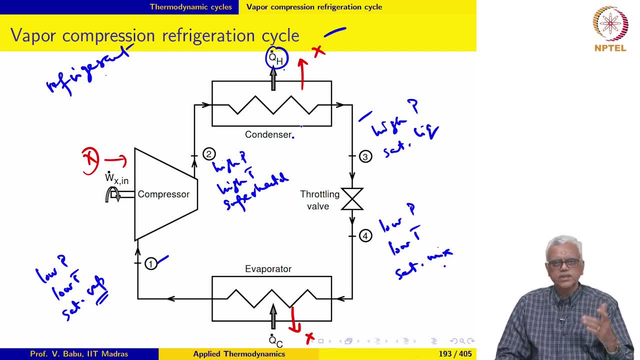 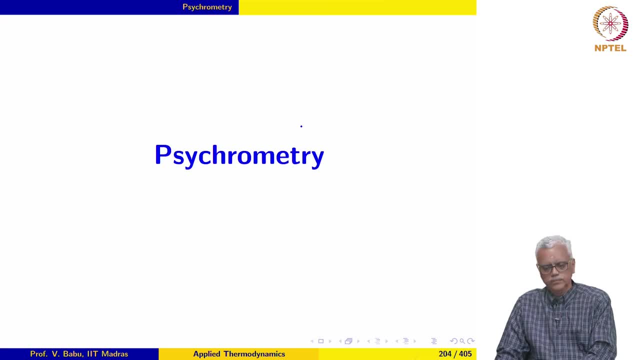 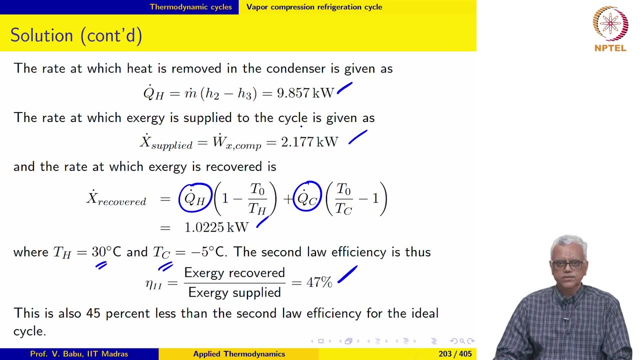 properties and so on are also being developed, But these are usually discussed in the next level course on refrigeration and air conditioning. So this concludes our lectures on thermodynamic cycles, where we looked at Rankine cycle, air standard cycles, within which we discussed 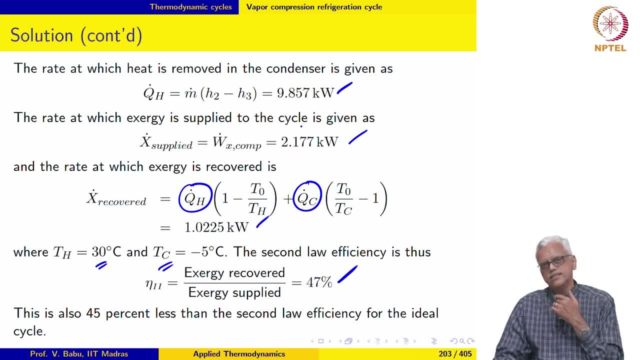 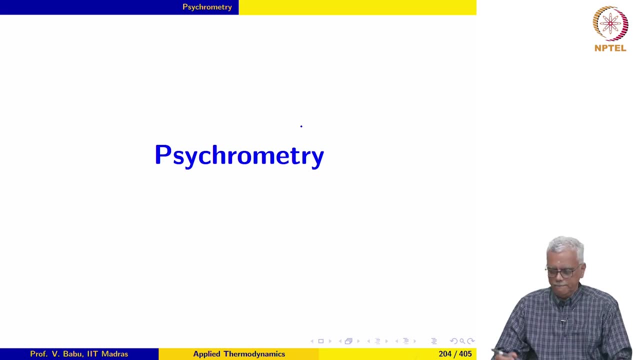 Air standard cycles, standard Brayton cycle, air standard auto and air standard diesel cycle, and then vapor compression refrigeration cycle, which is the only power absorbing cycle among all these cycles. The next module that we will take up is psychrometry.